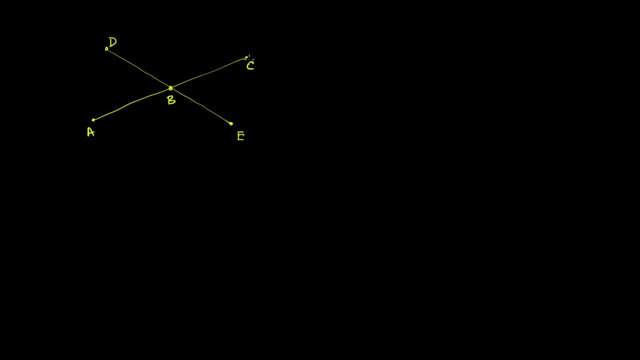 It looked like an F. This is angle CBE. What I want to do is, if I can prove that angle CBE is always going to be equal to its vertical angle, so angle DBA, then I prove that vertical angles are always going to be equal, because this is just a generalizable case. 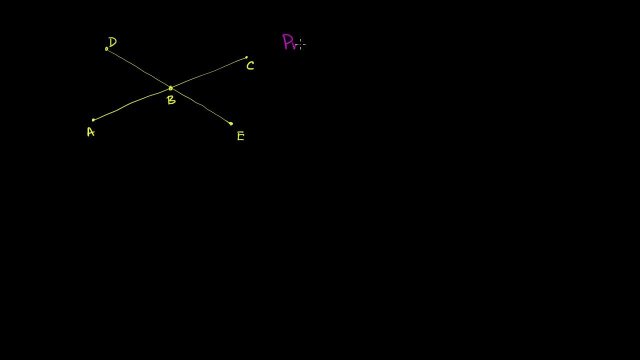 right over here. So what I want to prove here is angle CBE is equal to, I could say, the measure Of angle CBE. You'll see it's different ways. Actually, this time let me write it without measure so that you get used to the different notations. 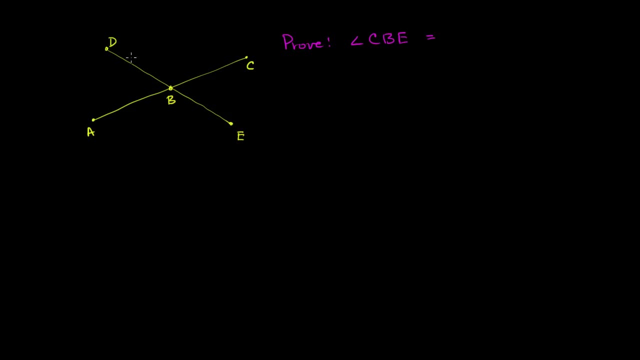 I'll just say: prove: angle CBE is equal to angle DBA. So the first thing we know. so what do we know? We know that angle CBE and we know that angle DBC are supplementary. They are adjacent angles And their outer sides of both angles. 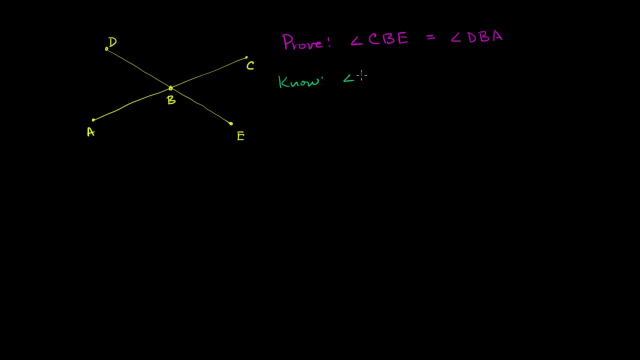 form a straight angle over here. So we know that angle CBE and angle DBC are supplementary. I'll just write sup for that. They're supplementary, which means that angle CBE plus angle DBC is equal to 180 degrees. Fair enough. 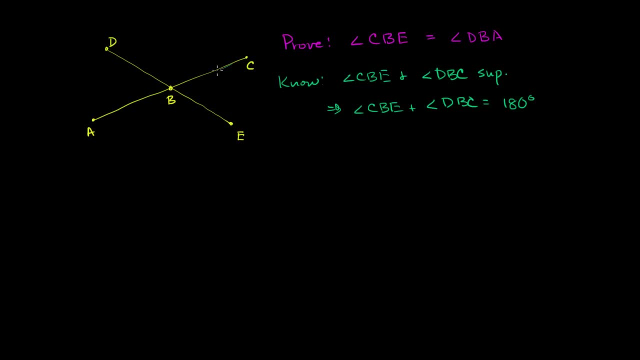 Fair enough, We also know. so let me see, This is CBE, This is what we care about, And we want to prove that this is equal to that. We also know that angle DBA. we know that this is DBA right over here. 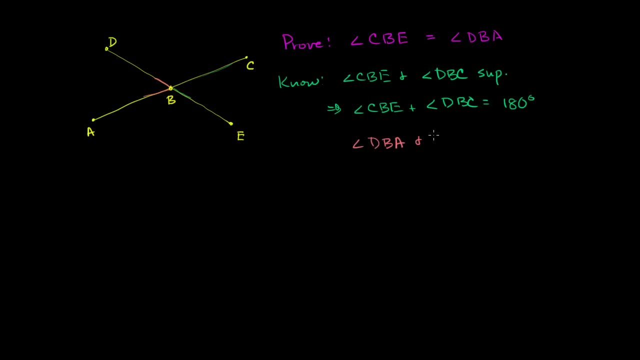 We also know that angle DBA and angle DBC are supplementary. This angle and this angle are supplementary. Their outer sides form a straight angle, They are adjacent, So they are supplementary, which tells us that angle DBA, this angle right over here, plus angle DBC. 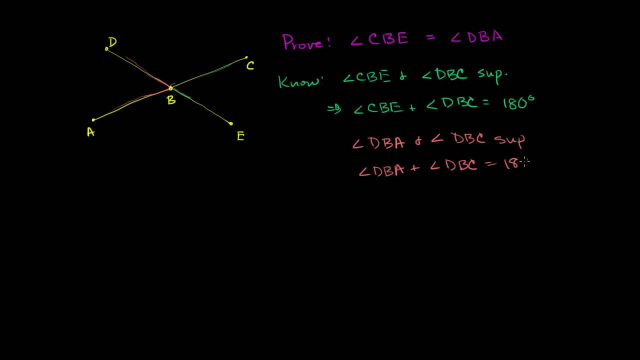 this angle over here is going to be equal to 180 degrees. Now from this top one, this top statement over here, we can subtract angle DBC from both sides And we get angle CBE is equal to 180 degrees. So angle DBA is equal to 180 degrees, minus angle DBC. 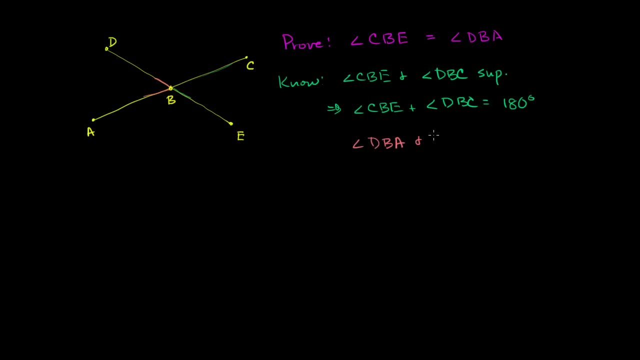 We also know that angle DBA and angle DBC are supplementary. This angle and this angle are supplementary. Their outer sides form a straight angle, They are adjacent, So they are supplementary, which tells us that angle DBA, this angle right over here, plus angle DBC. 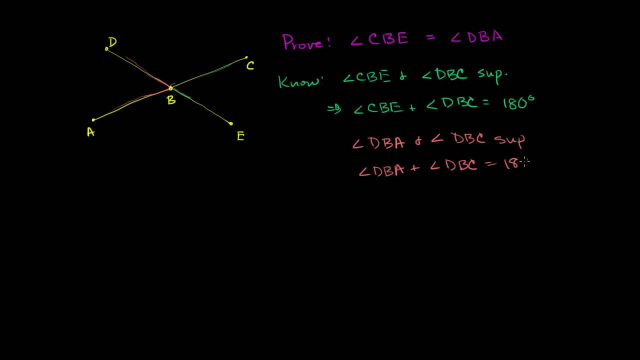 this angle over here is going to be equal to 180 degrees. Now from this top one, this top statement over here, we can subtract angle DBC from both sides And we get angle CBE is equal to 180 degrees. So angle DBA is equal to 180 degrees, minus angle DBC. 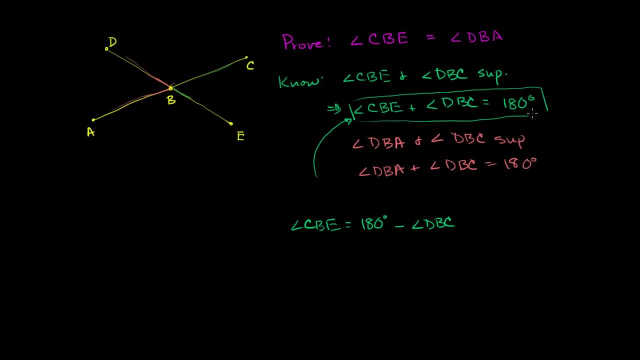 That's this information right over here. I just put the angle DBC on the right side, or I subtracted it from both sides of the equation, And this right over here. if I do the exact same thing- subtract angle DBC from both sides of the equation. 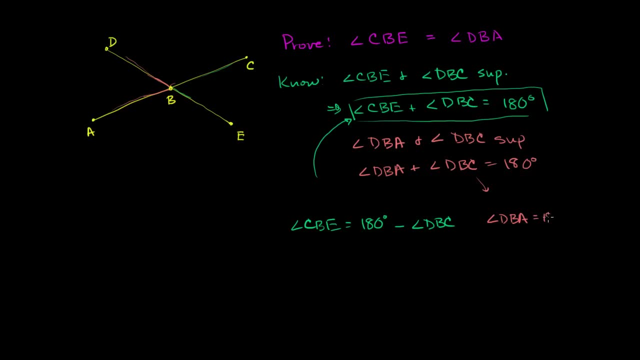 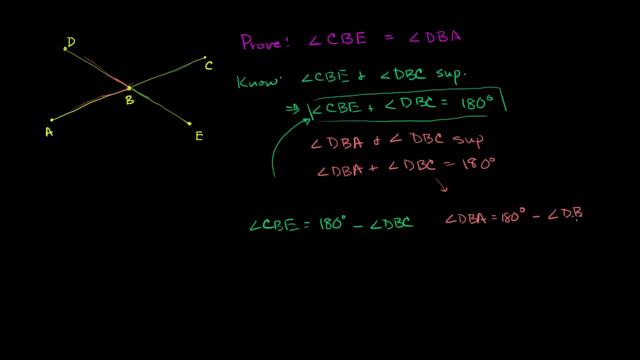 I get. angle DBA is equal to 180 degrees. Let me scroll over to the right a little bit. Is equal to 180 degrees minus angle DBC. So clearly, angle CBE is equal to 180 degrees minus angle DBC. 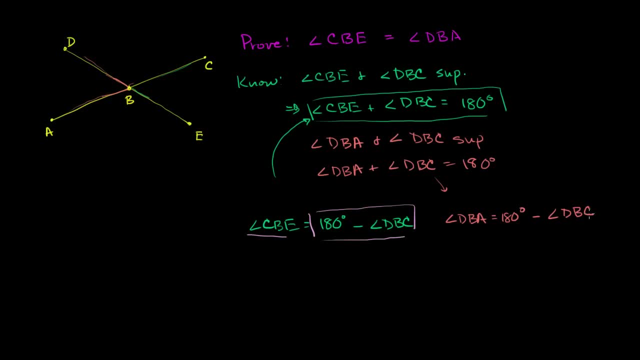 Angle DBA is equal to 180 degrees minus angle DBC, So they are equal to each other. They are both equal to the same thing. So we get which is what we wanted to get. angle CBE is equal to angle DBA. 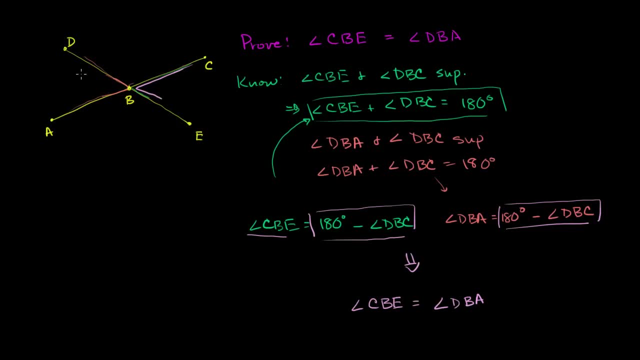 Angle CBE, which is this angle right over here, is equal to angle DBA, And sometimes you might see that shown like this. So angle CBE- that's its measure, And you'd say that this measure right over here is the exact same amount. 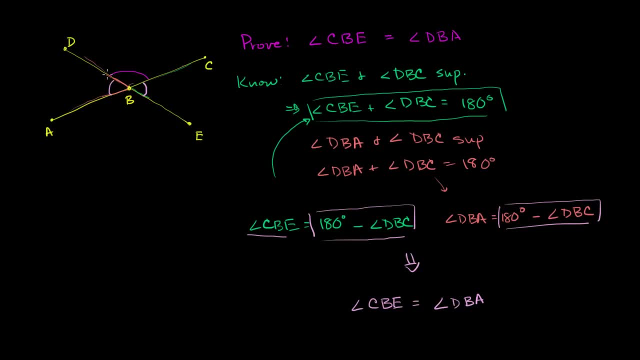 And we have other vertical angles. Whatever this measure is- and sometimes you'll see it with a double line like that- you could say that that is going to be the same as whatever this angle right over here is. You'll see it written like that sometimes. 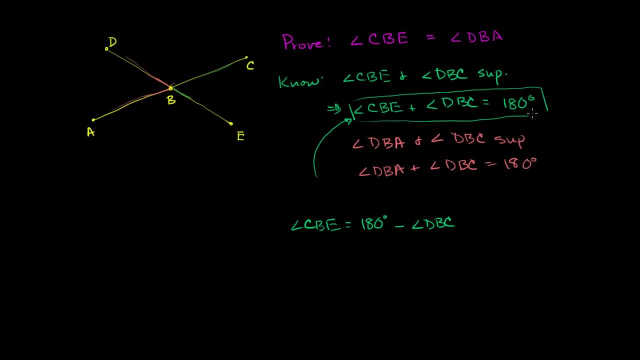 That's this information right over here. I just put the angle DBC on the right side, or I subtracted it from both sides of the equation, And this right over here. if I do the exact same thing- subtract angle DBC from both sides of the equation. 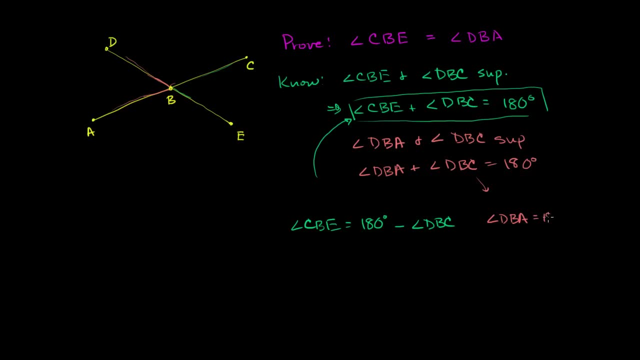 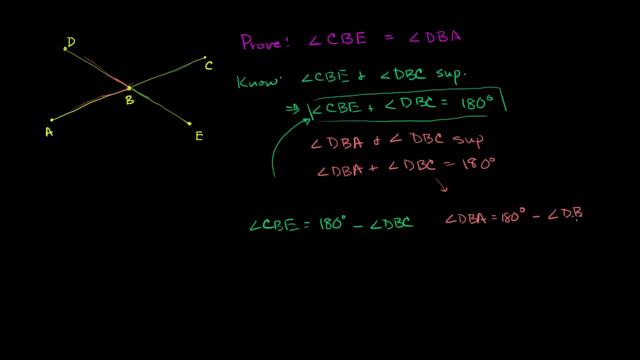 I get. angle DBA is equal to 180 degrees. Let me scroll over to the right a little bit. Is equal to 180 degrees minus angle DBC. So clearly, angle CBE is equal to 180 degrees minus angle DBC. 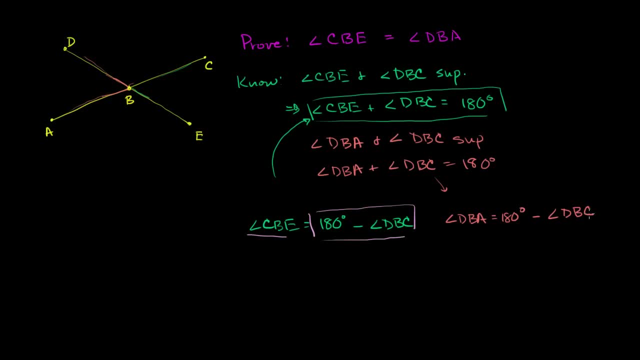 Angle DBA is equal to 180 degrees minus angle DBC, So they are equal to each other. They are both equal to the same thing. So we get which is what we wanted to get. angle CBE is equal to angle DBA. 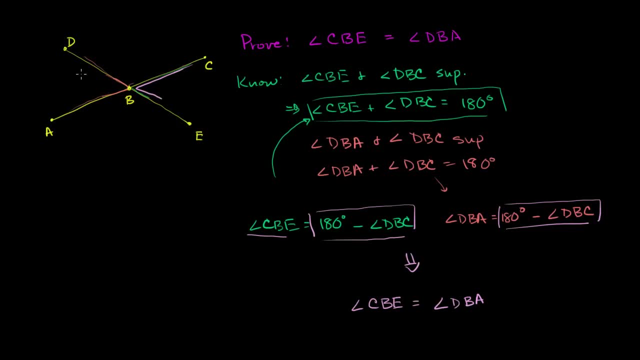 Angle CBE, which is this angle right over here, is equal to angle DBA, And sometimes you might see that shown like this. So angle CBE- that's its measure, And you'd say that this measure right over here is the exact same amount. 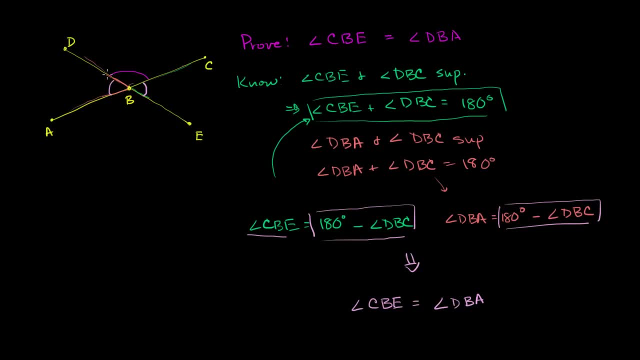 And we have other vertical angles. Whatever this measure is- and sometimes you'll see it with a double line like that- you could say that that is going to be the same as whatever this angle right over here is. You'll see it written like that sometimes. 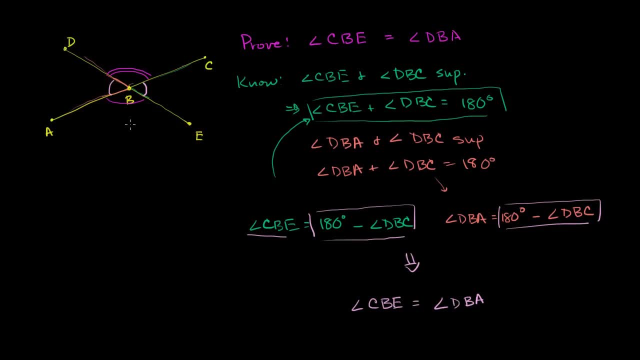 I like to use colors, but not all books have the luxury of colors, Or sometimes you'll even see it written like this: to show that they're the same angle- This angle and this angle- and show that these are different. Sometimes they'll say that they're the same in this way. 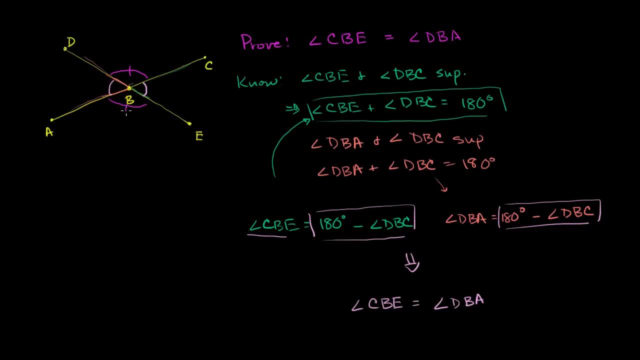 This angle is equal to this vertical angle, is equal to its vertical angle right over here, And this angle is equal to this angle. that's opposite the intersection right over here. But we've proved it for the general case, Because all I did here is I just did. 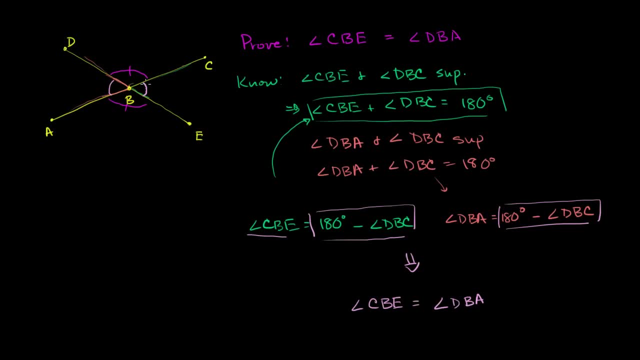 two general intersecting lines. I picked a random angle and then I proved that it's equal to the angle that is vertical to it.